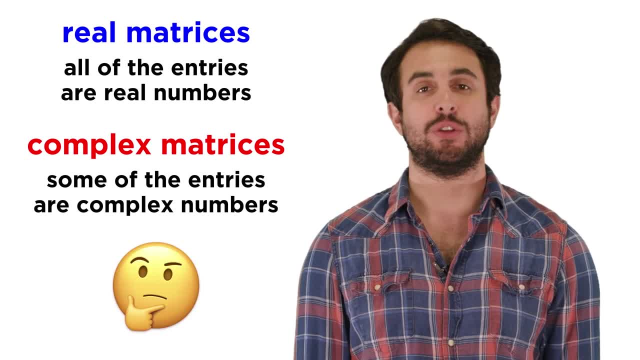 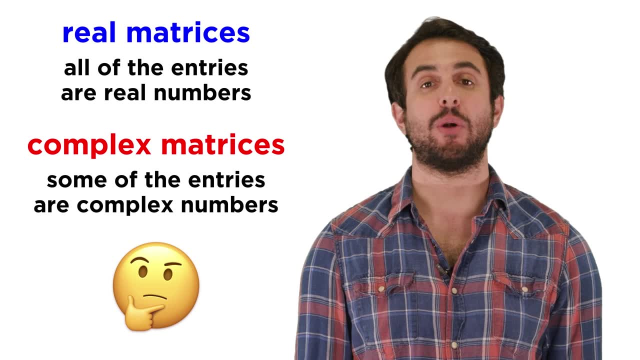 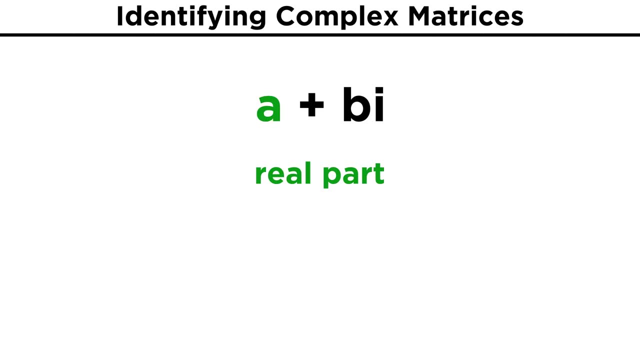 contain complex numbers. If you need a little review regarding complex numbers, what they are and relevant operations, check out this tutorial from earlier in the series. Otherwise, let's dive right in. We can simply recall that complex numbers are numbers with a real part A and an imaginary. 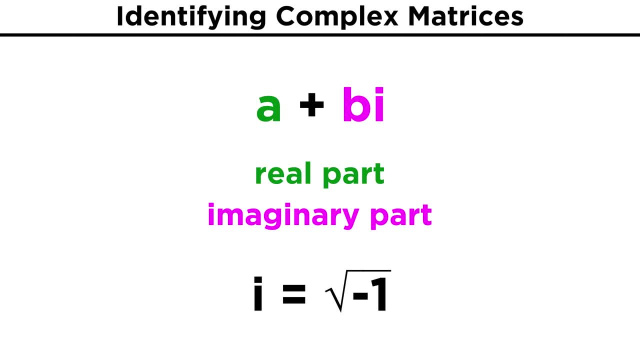 part B, I, where I is the square root of negative one. and, as we said, we can find complex numbers in matrices. Just the way we can separate complex numbers into a real component and an imaginary component, we can separate matrices into a real matrix. 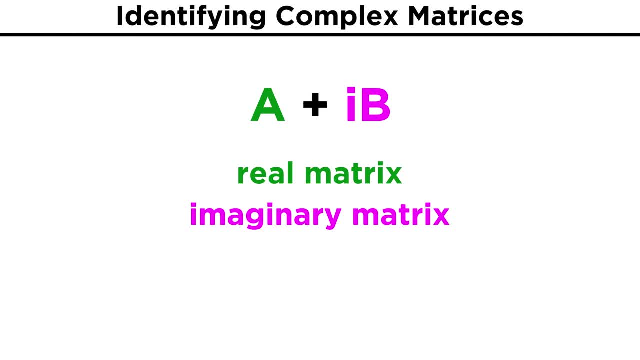 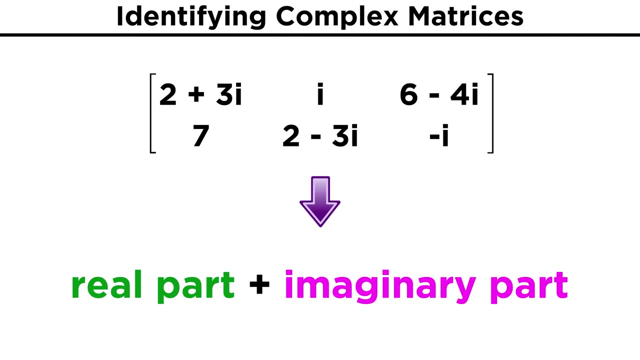 A and an imaginary matrix I B. For example, let's consider the two by three matrix: two plus three I I. six minus four, I seven. two minus three, I, negative I. We can split this complex matrix up into a real part plus an imaginary part, by keeping in mind that: 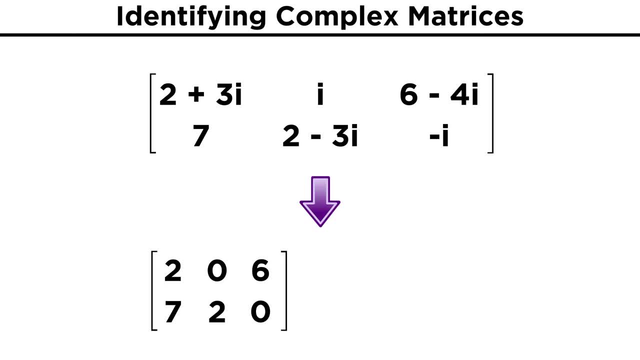 matrix addition works element by element. First, for the real part, we just take the real part of each element and put them in a matrix of the same size. So for the first entry, we take the two from two plus three. I Continuing in this manner. 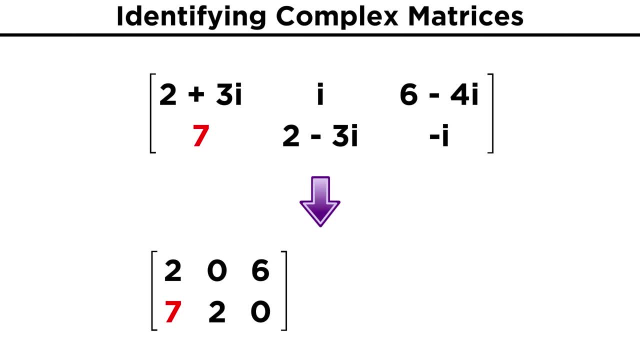 will give us two zero, six, seven, two zero. Then we do this again for the imaginary part of each element. so this time we take the three I from two plus three I. That will give us I times three, one negative four zero negative three negative one. 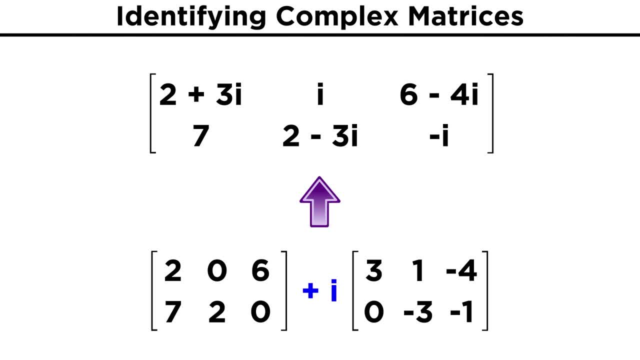 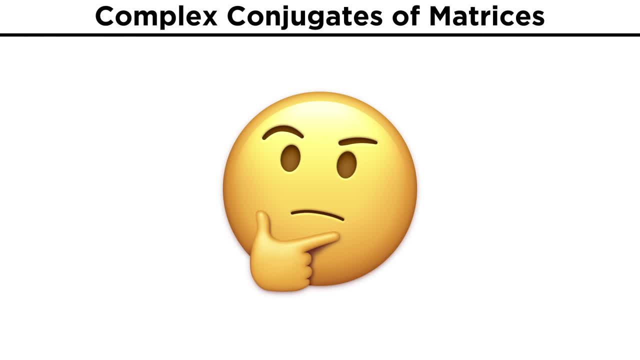 We could distribute the I and add the two matrices together to get what we started with. Now that we know what complex matrices are, we must consider the complex conjugates of matrices. Recall that for ordinary complex numbers we learned that the complex conjugate is the. 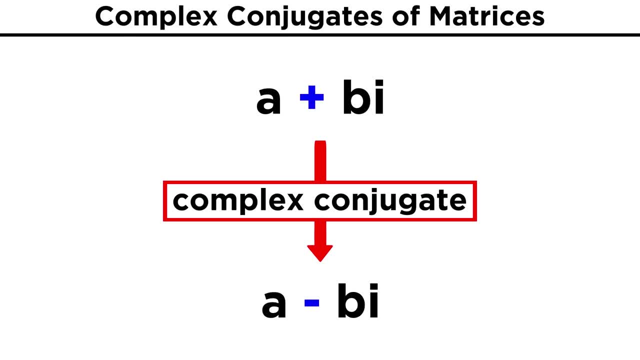 same as switching the sign on the imaginary term. so A plus B I would become A minus B I. Similarly, the conjugate of a complex matrix, A plus IB, is simply A minus IB. We actually don't even have to take the step of splitting up the real and complex. 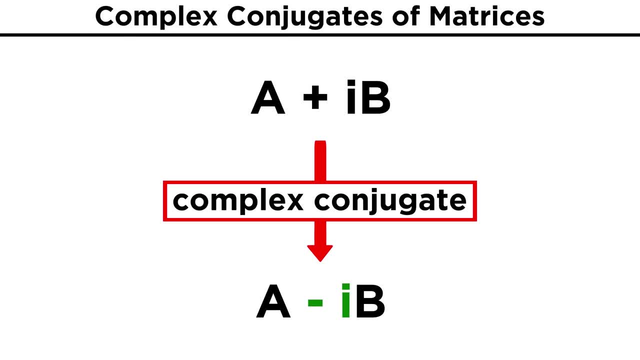 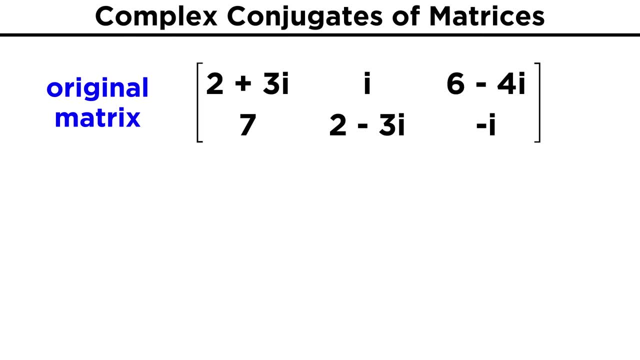 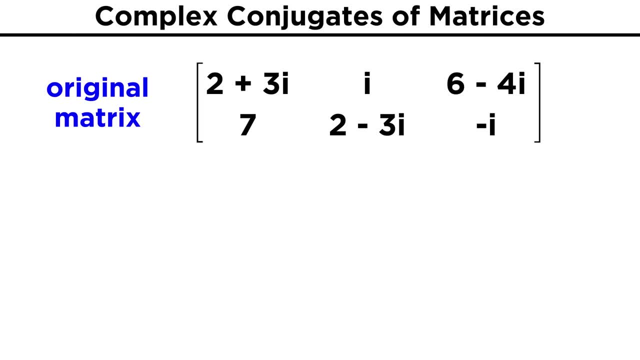 i six minus four, i seven. two minus three. i negative i. the conjugate will be two minus three, i negative. i six plus four, i seven, two plus three, i i. So this is certainly simple enough. however, when it comes to matrices, there is another. 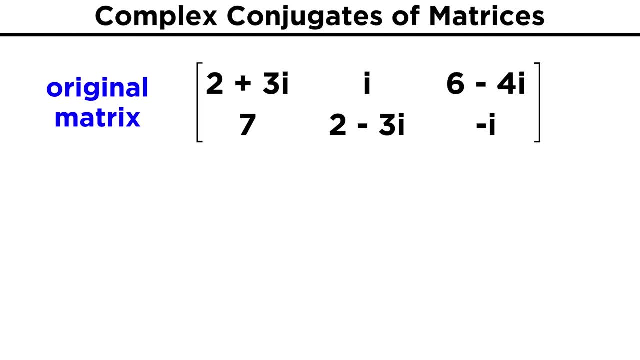 operation that is much more important than taking the conjugate, and this is taking the conjugate transpose. Finding this is not too difficult: you simply take the conjugate, as we just did, and then take the transpose of the matrix, which, as we recall, involves making the columns into 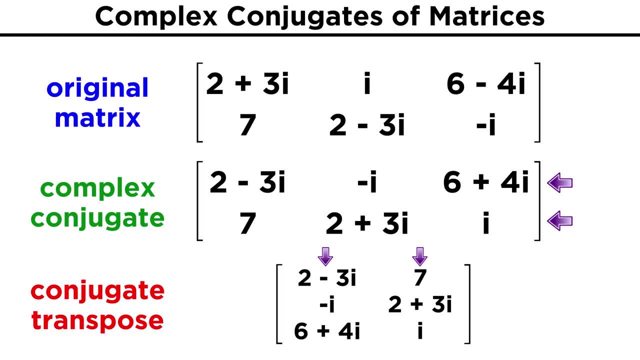 rows and the rows into columns. The reason we want to do this is so that we can multiply the matrix and the conjugate. transpose Simply taking the conjugate will not give us matrices we can multiply. For example, our two by three matrix cannot be multiplied by its two by three conjugate. 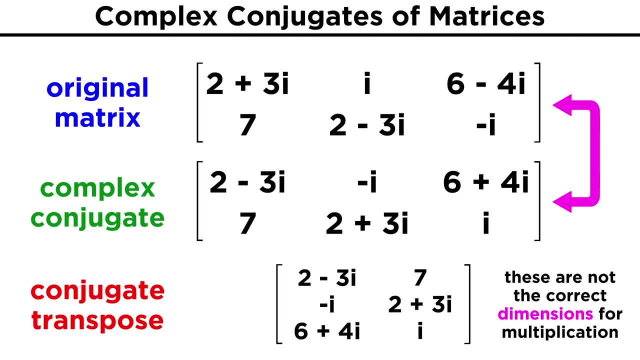 because of the way matrix multiplication works, which we recall from a previous tutorial. But if we take the transpose of the conjugate, we will get a three by two matrix and now we can multiply them with no problem. We've already seen that the conjugate was two minus three, i negative, i six plus four. 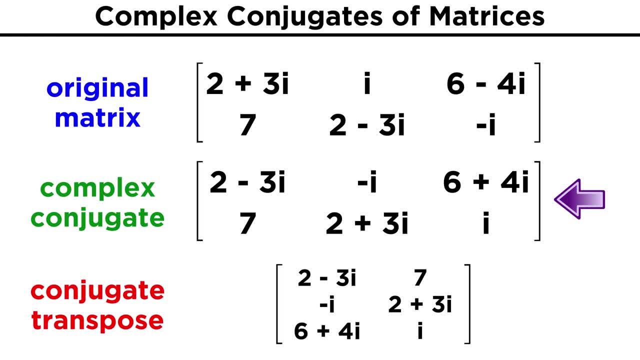 i seven, two plus three i i. So, taking the transpose, we will get two minus three i seven, negative i, two plus three i six plus four i i. This is our conjugate transpose, also referred to as the Hermitian transpose. 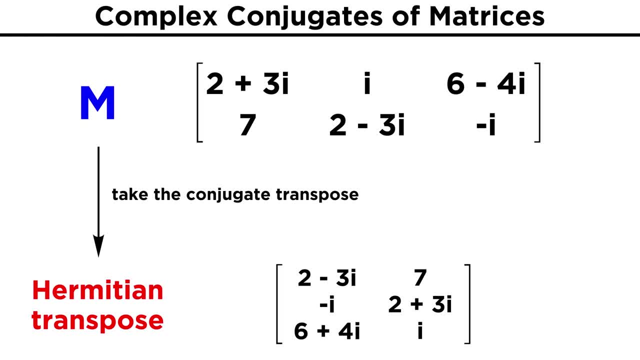 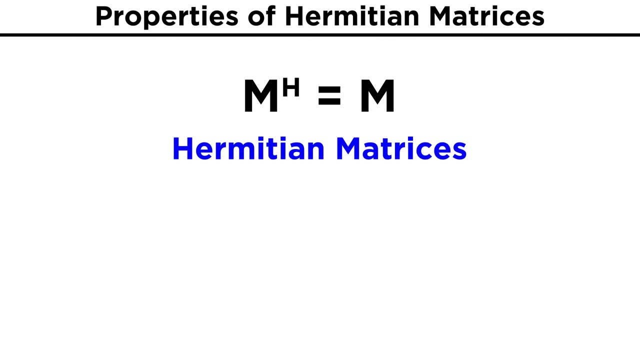 Given a matrix M. the notation for taking the conjugate transpose is MH, Or in some fields an M, with this symbol read as M dagger. Now that we understand the conjugate transpose, let's look at a special type of matrix called. 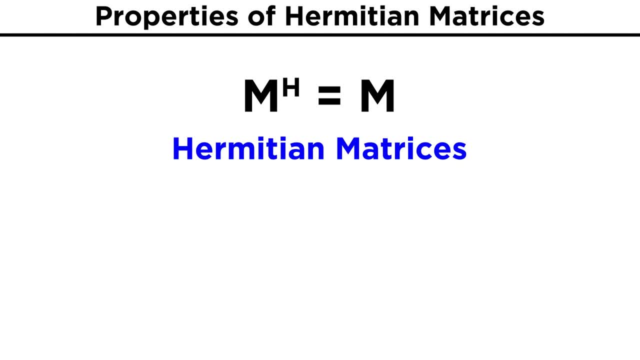 Hermitian matrices. These are square matrices whose conjugate transpose is the same as the original matrix. For example, consider the matrix two, one minus i, one plus i three. Taking the conjugate first, we get two, one plus i, one minus i, three. 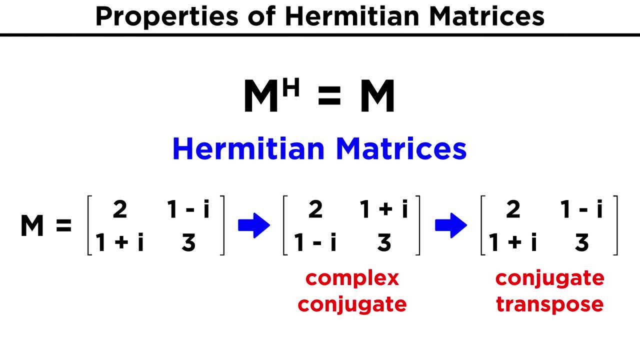 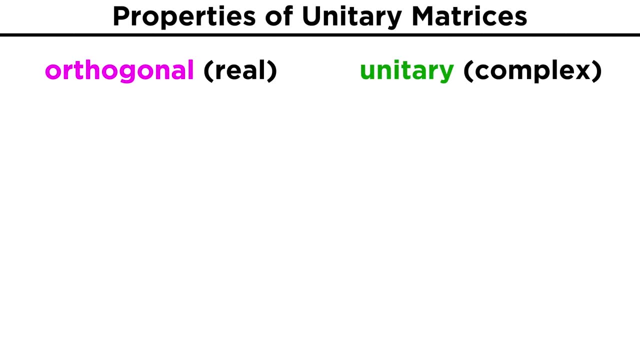 Now, taking the transpose, we end up with two, one minus i, one plus i three, which is precisely the matrix we started with meaning. this matrix is Hermitian. Finally, recall two things. First, that real matrices are considered orthogonal if the column is orthogonal. 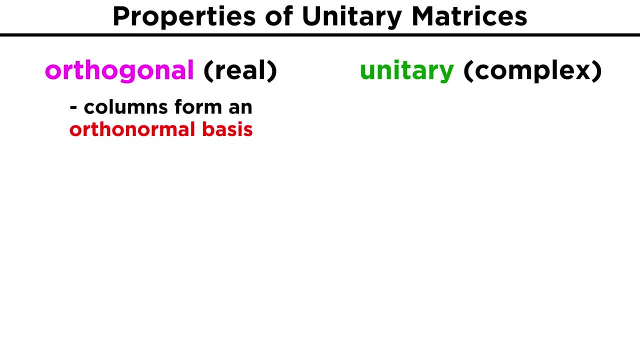 So if the column is orthogonal, then the matrix is Hermitian. If the column is orthogonal, then the matrix is Hermitian. Second, that the columns form an orthonormal basis. And second, that the inverse of an orthogonal matrix is the same as its transpose. 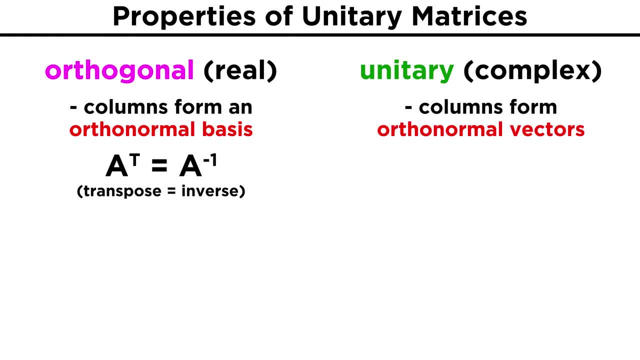 For complex matrices, if the columns form orthonormal vectors, the matrix is said to be unitary and the conjugate transpose of the matrix is the same as the inverse of the matrix. It's worth noting that a real unitary matrix is just an orthogonal matrix. 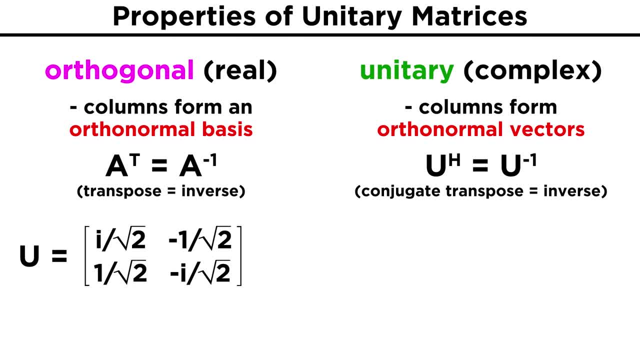 Let's consider the matrix: U equals i over root two. negative. one over root two. one over root two negative i over root two. To check if this is unitary, we can simply take the conjugate, transpose UH and see: 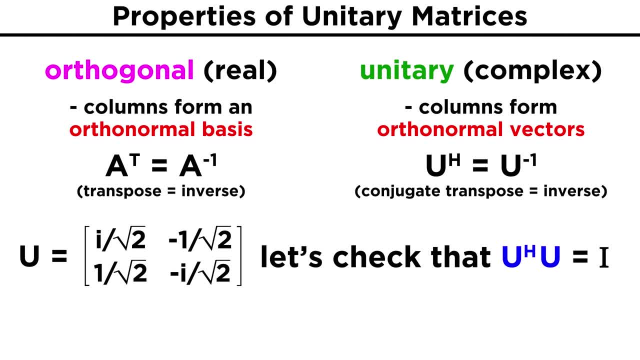 if UH times U gives the identity matrix, The conjugate of U will be negative: i over root two. negative. one over root two. one over root two. i over root two. Then, taking the transpose, we get UH equals negative. i over root two. one over root two. 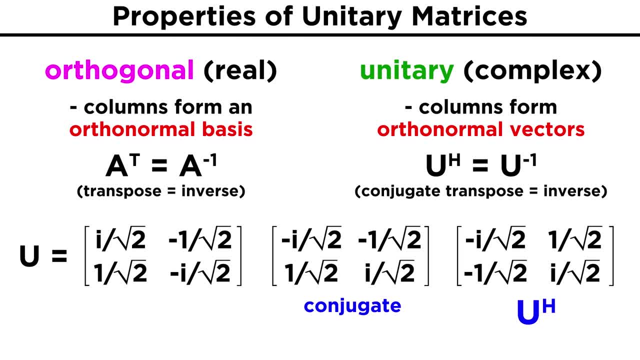 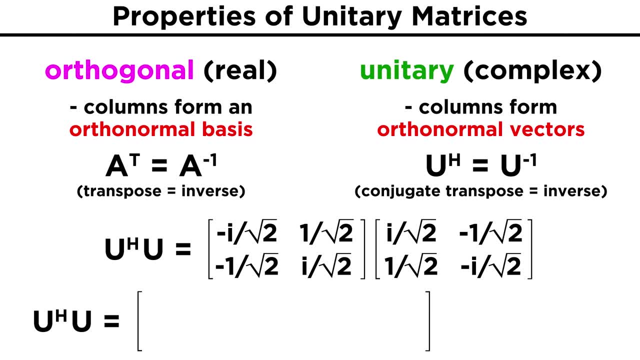 negative: one over root two: i over root two. We will now multiply UH and see what we get. Doing the matrix multiplication. we get negative: i squared over two plus one half i over two minus i over two. Negative: i over two plus i over two. one half minus. i squared over two.